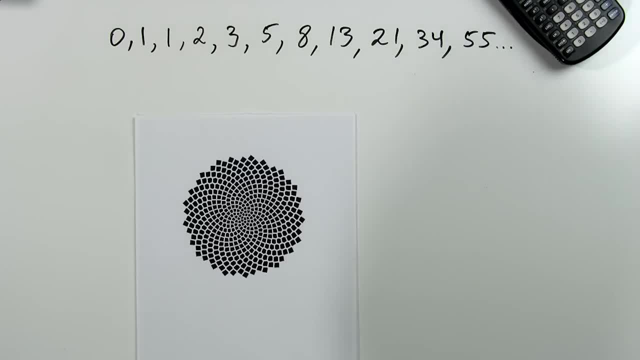 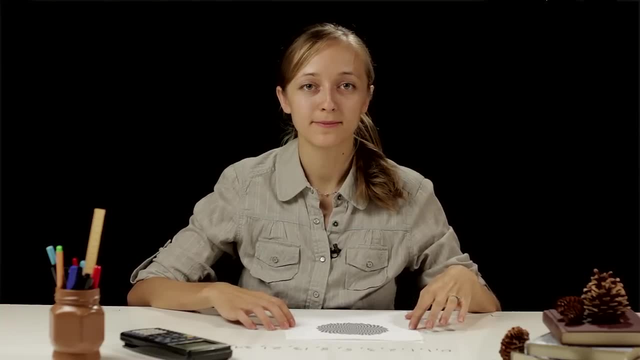 find that there are multiple spirals here in different directions. If this is a true Fibonacci pattern, then the number of spirals when added up will always be a Fibonacci number. For example, if we count the number of spirals going in this direction, we will find that 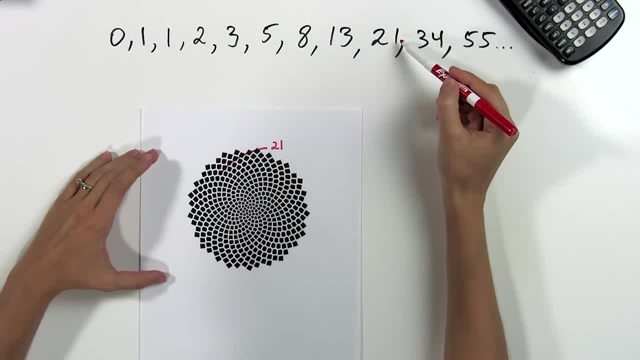 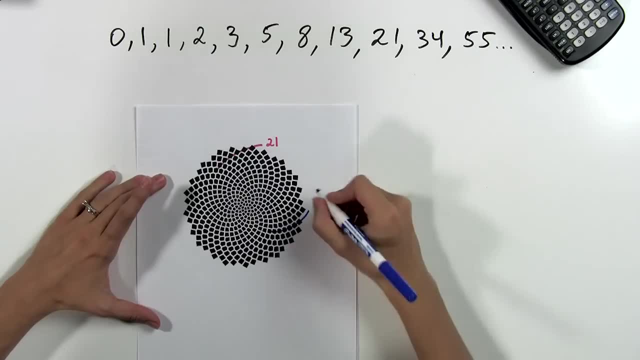 there are 21 of them when we add them up, And 21 is one of our numbers. Or we could count the spirals going in this direction, in which case we would get 34 total spirals, And that, of course, is also one of our numbers. 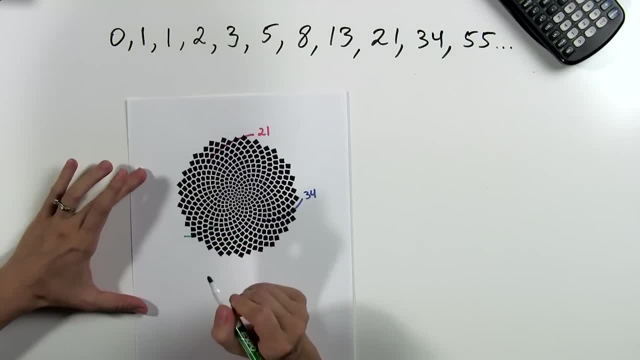 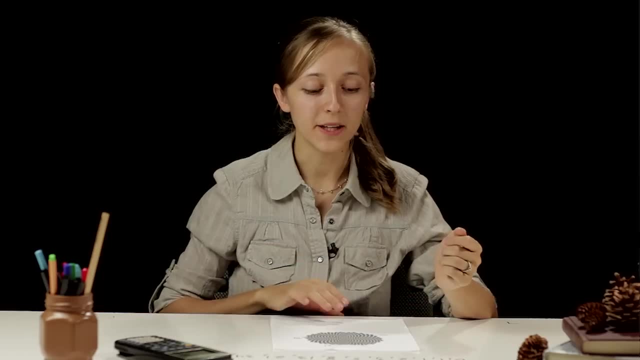 Or there is a third way we could count it going this way, in which case we would get 55 total spirals, which is also one of our numbers. Now that you know what a Fibonacci spiral is and what it looks like, take a look at. 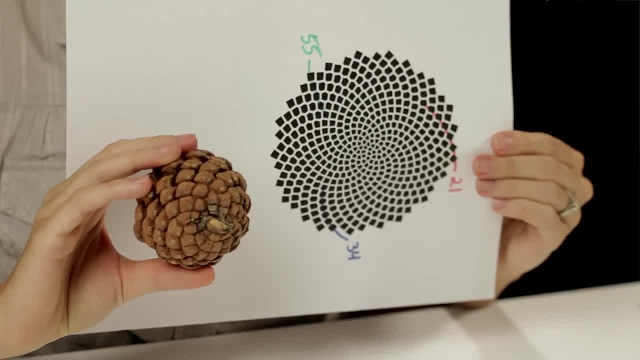 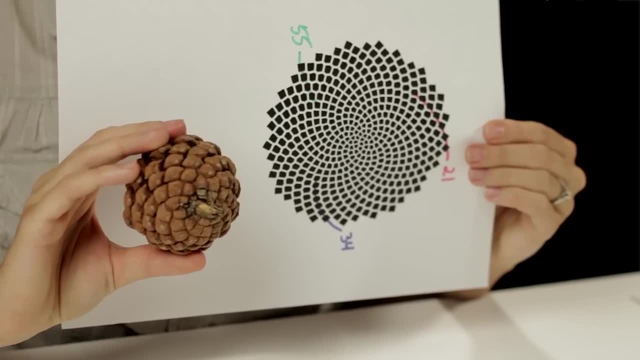 this pine cone. Do you see how it resembles the same spirals? The same is true of almost all pine cones. If you count their spirals in any direction, you will get a Fibonacci number. Another way that Fibonacci numbers appear in nature is in the way animals reproduce. 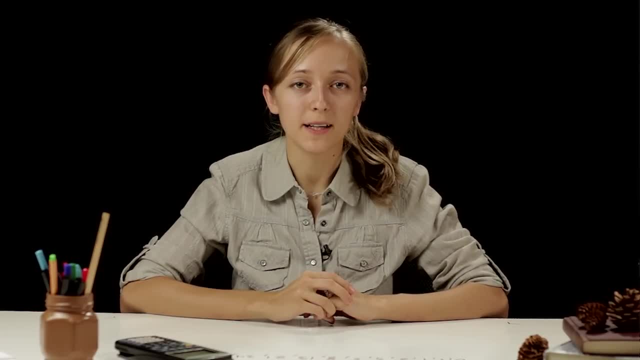 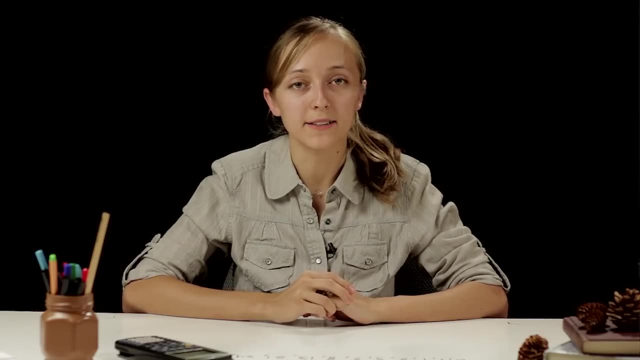 like rabbits and honey bees. For example, if a female honey bee lays an egg and it is unfertilized, then a male will hatch, so each male bee has only one parent. If the egg is fertilized, then a female will hatch, so all female bees have one parent. 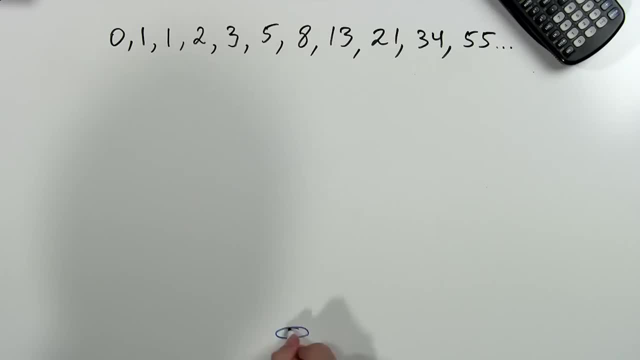 Now, let's imagine one male bee. Since he's a male, he has only one parent, a female. Since this is a female, she has two parents, a female and a male. This female also has two parents. This female has two parents. 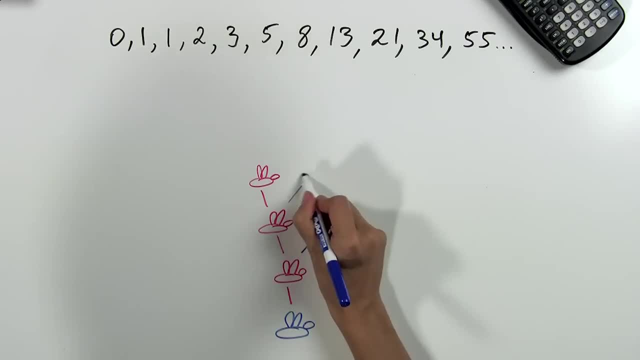 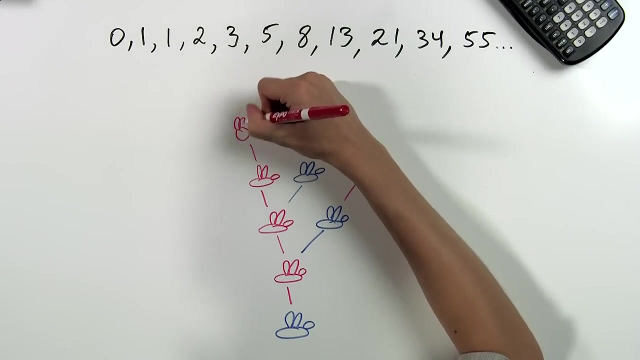 This female has two parents. This female has two parents, But this male only has one. Let's do one more row of parents. This female has a female and a male parent. This male only has one female parent. This female has a male parent.